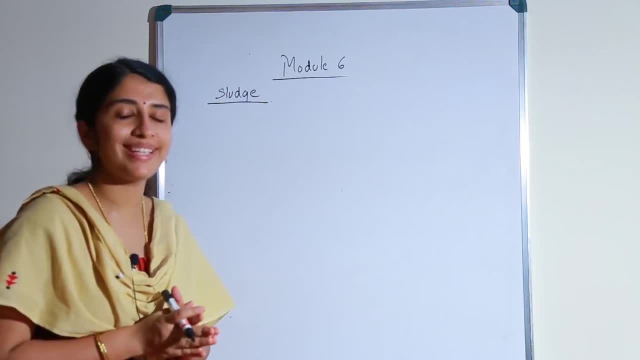 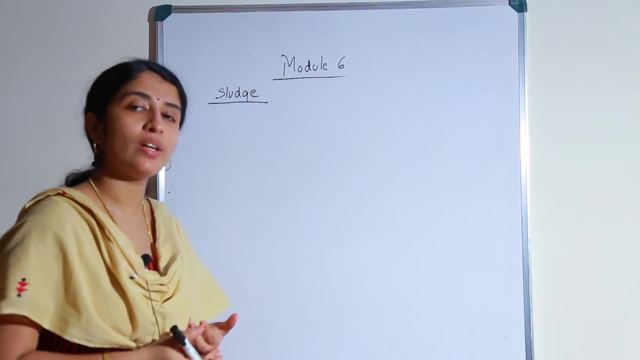 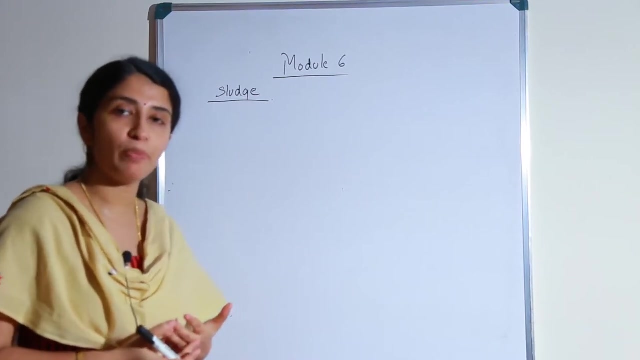 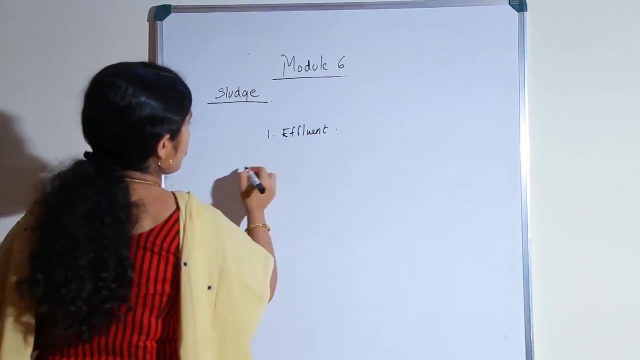 Hello students, today we are starting our module 6.. Module 6 is dealing with the sludge and various sludge treatment methods. So first let us see what is actually a sludge. We know that after a wastewater treatment we are getting two end products. The first one is effluent, which means the wastewater, treated wastewater. Then the second one is what you call as sludge. 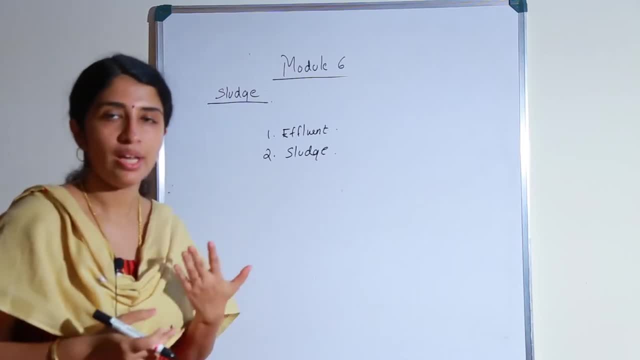 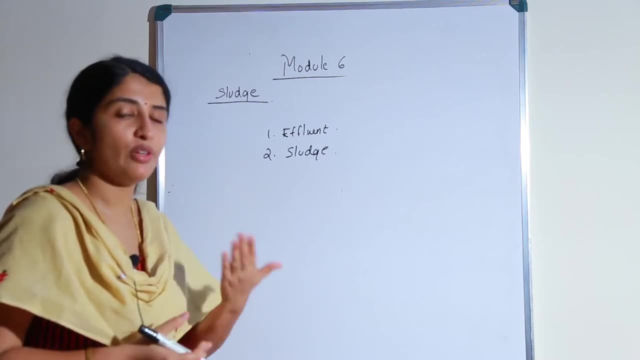 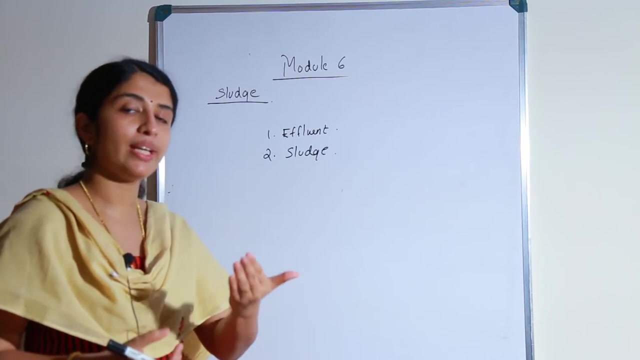 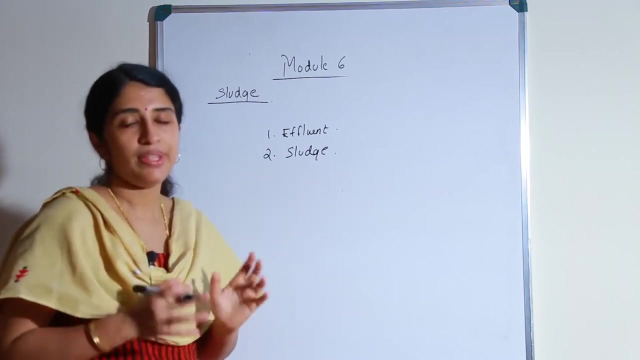 So these are the two end products of the wastewater treatment. So sludge means it is the settled particles in different wastewater system. If you are considering a primary sedimentation tank, you know that after the working of primary sedimentation tank the suspended particles will get settled down at the bottom. That settled particles is called as sludge. The peculiarity of this sludge is that it is having high amount of organic matter. 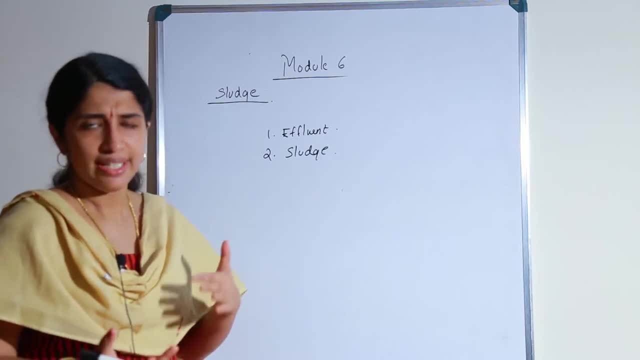 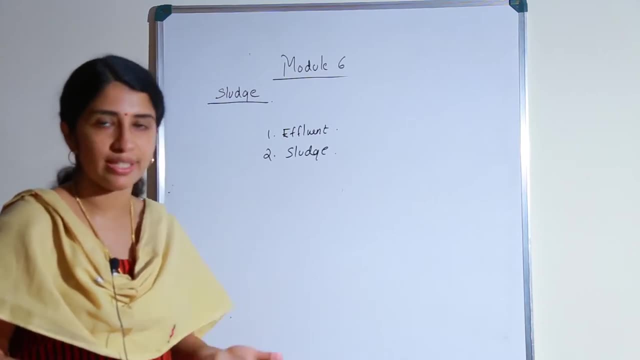 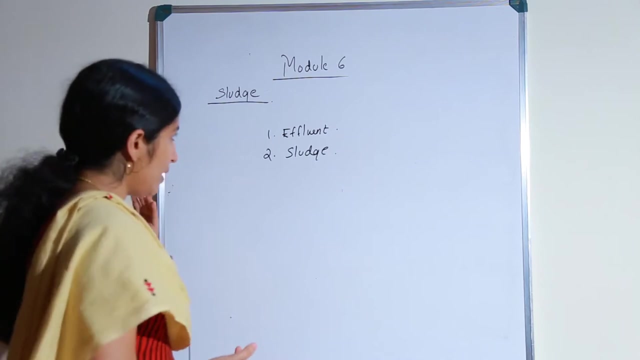 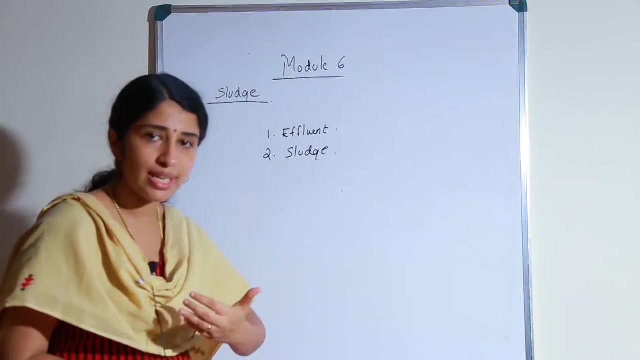 And also it is having high amount of moisture content. Since it is highly, it is containing high amount of organic matter, it is highly purchasable in nature or offensive in nature. So we have to treat it before the disposal. We know that when we are considering a wastewater treatment system, the wastewater is entering to different stages of treatment: from primary stage- primary treatment- then towards secondary treatment, then towards final tertiary treatment. 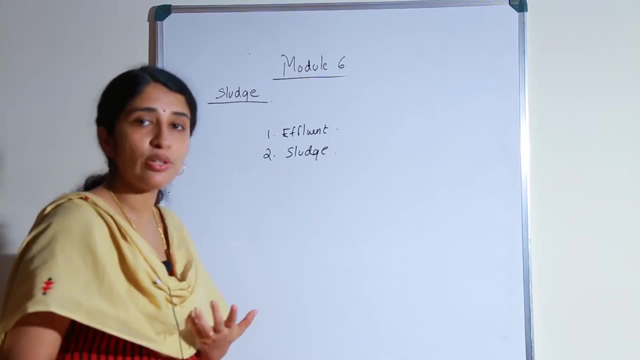 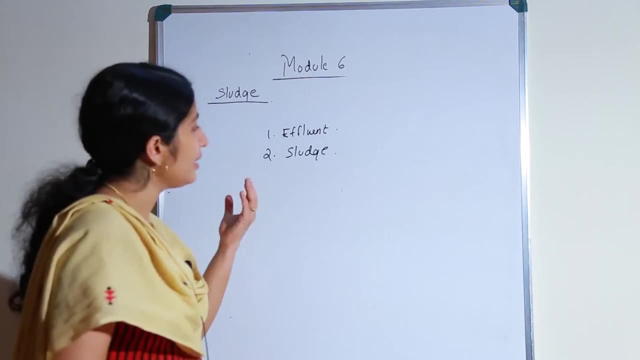 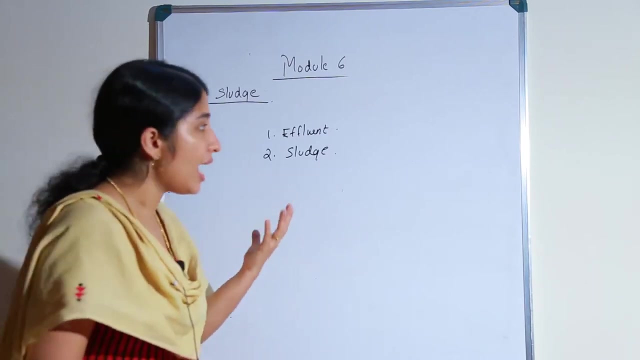 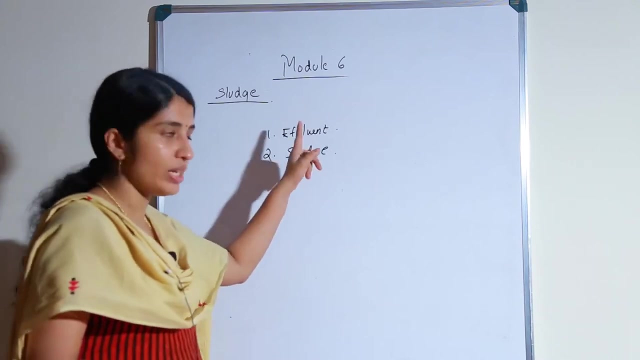 Or final disposal. But in each of the system, like primary sedimentation tank, activated sludge treatment process or a secondary settling tank, there exist the settled sludge at the bottom of this particular treatment system, So that sludge has to be treated before disposal, Just like the effluent or the treated wastewater. sludge is also having a great concern. It is having a great concern. 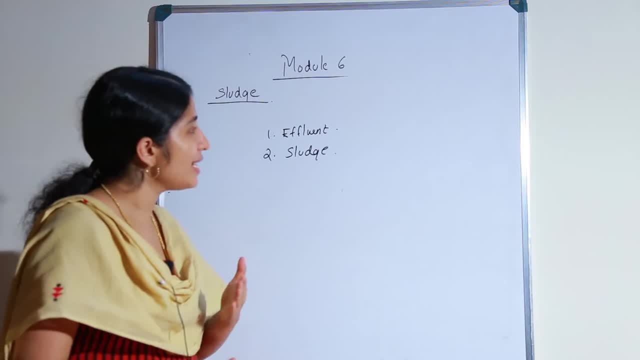 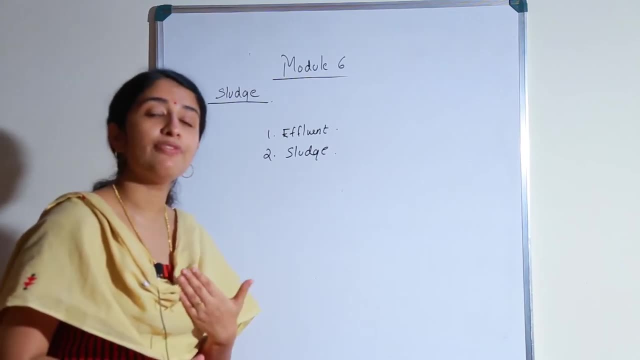 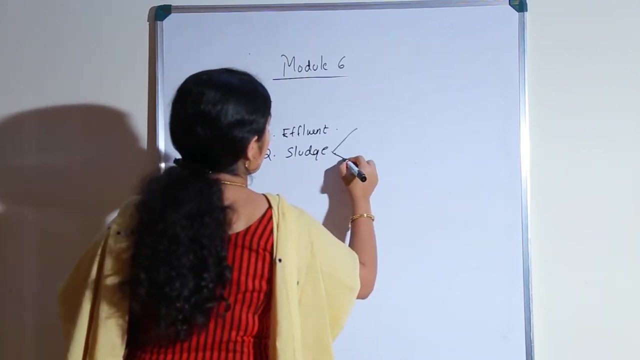 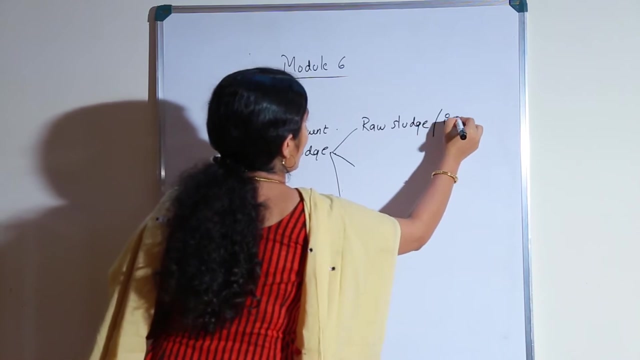 It is having a high amount of organic matter. So that is the need of the sludge treatment process. Before that, let us see what are the different types of sludges. Sludges are of three types. The first one is called raw sludge or primary sludge. 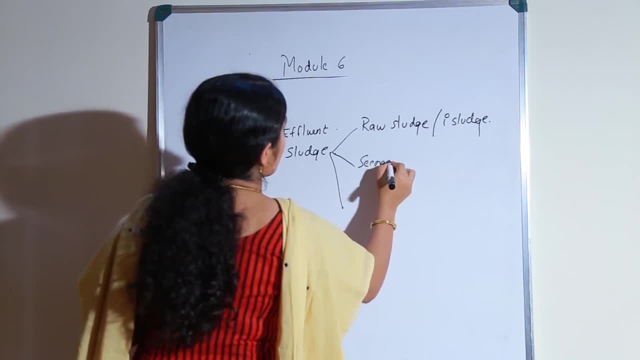 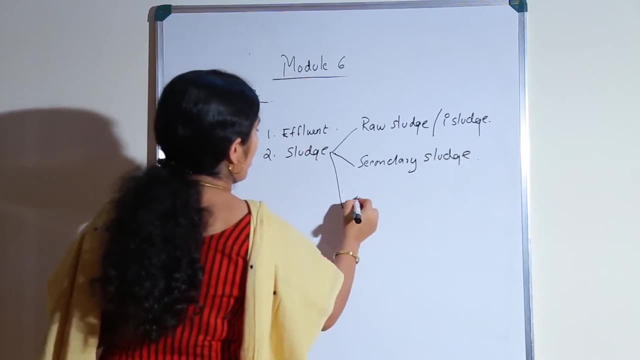 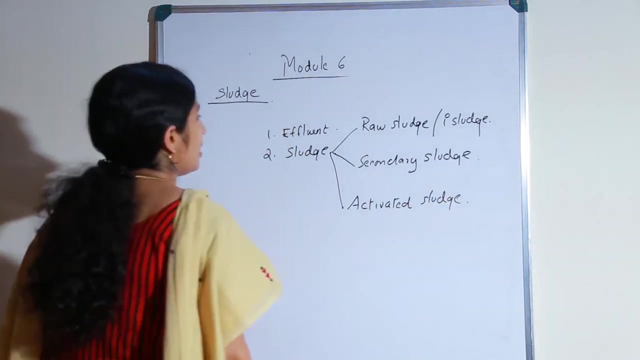 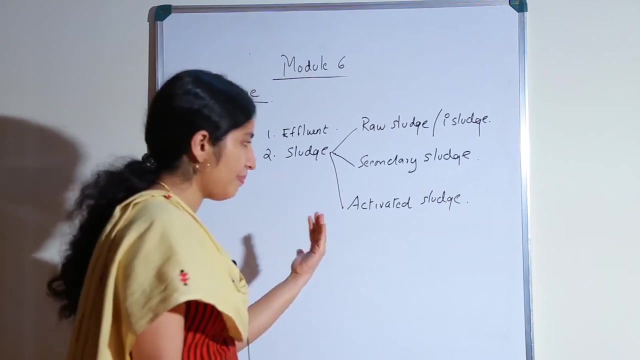 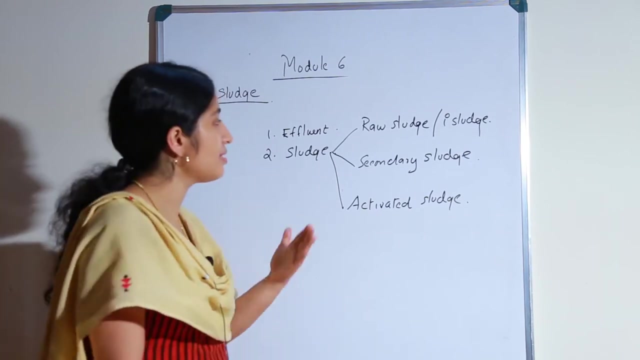 The second one is called secondary sludge. The third one is called activated sludge. This categorization or this different types are based on where the sludge occurs or what are the sources. of this is based on the sources of sludge. So this is based on the sources of sludge. 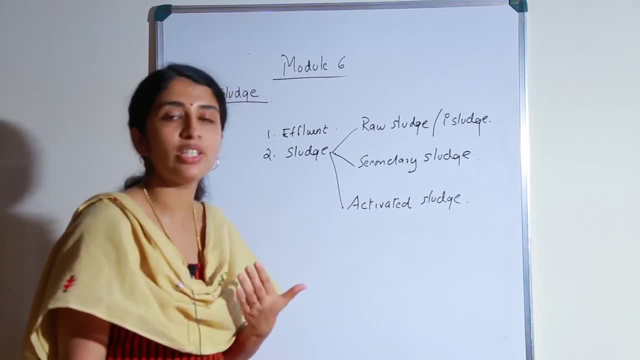 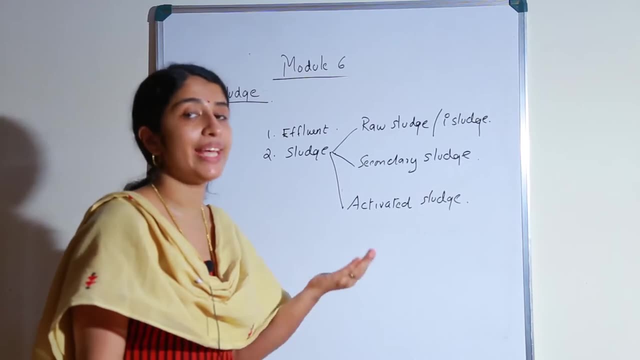 If we are taking the sludge from primary sedimentation tank, that sludge is known as raw sludge. If you are taking the sludge from the secondary sedimentation tank or a trickling filter, then that sludge is known as secondary sludge. 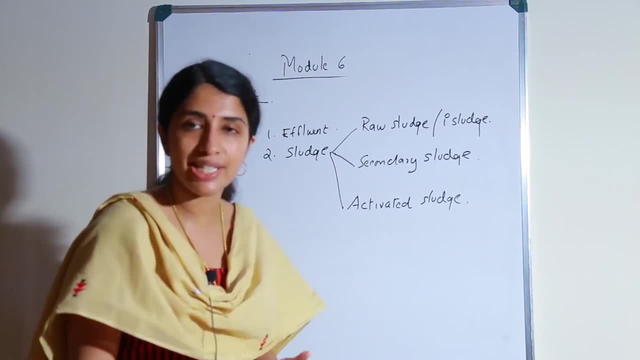 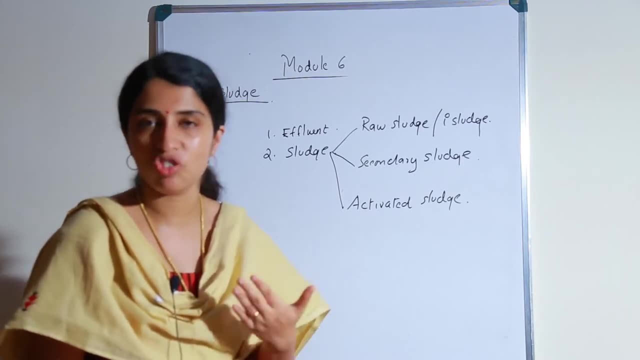 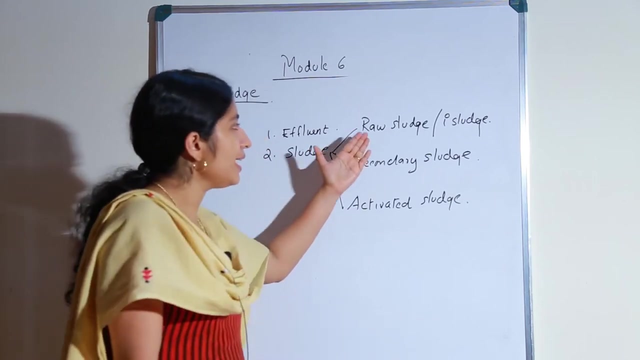 Activated sludge means it is the sludge deposited at the bottom of the sludge that we are getting from activated sludge treatment process. So this three are the three types, the different types of sledges in here in this three types, raw sludge contains really high. 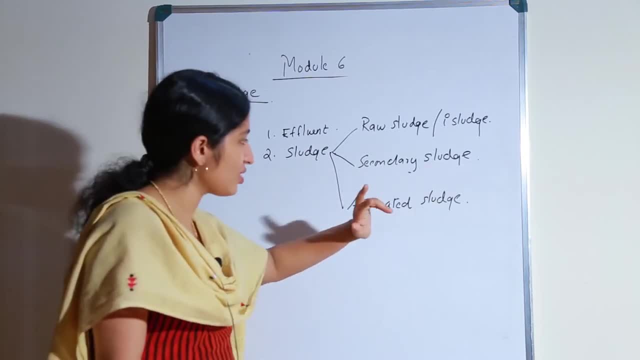 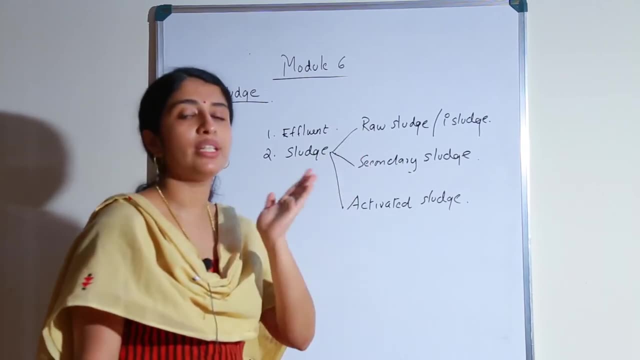 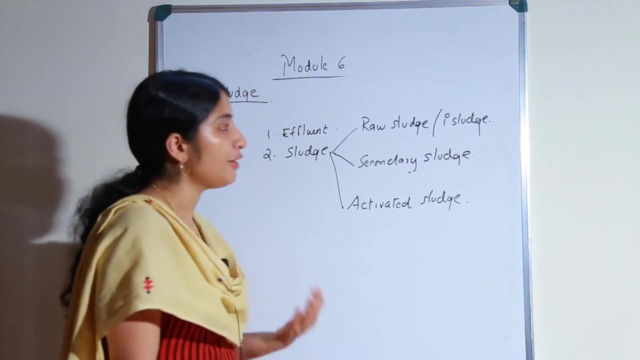 organic matter than the other two, that is, secondary sludge and activated sludge. so we have to treat the sludge before the disposal into a land or sea. so now we are going to see what are the different sludge treatment techniques used for the treatment process. 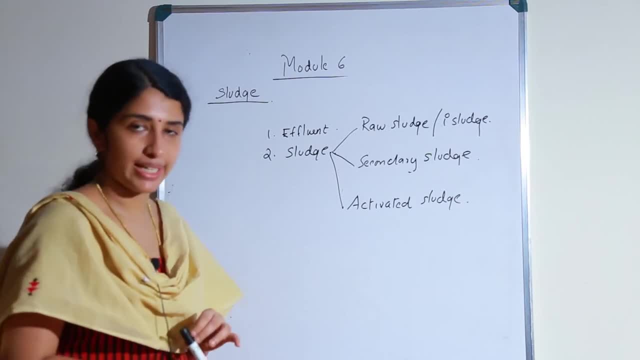 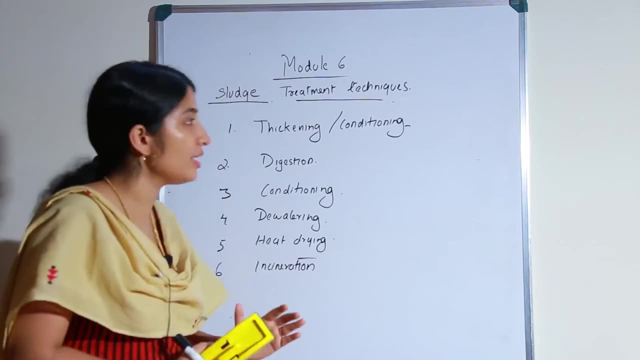 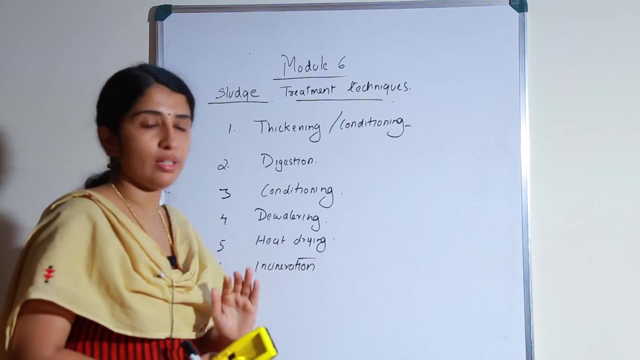 so let us see what are the different treatment techniques. these are the sludge treatment techniques that we are used. this is the order, or this is the flow chart, of sludge treatment process. the end, the general need or the general aim of these treatment techniques is to see what are. 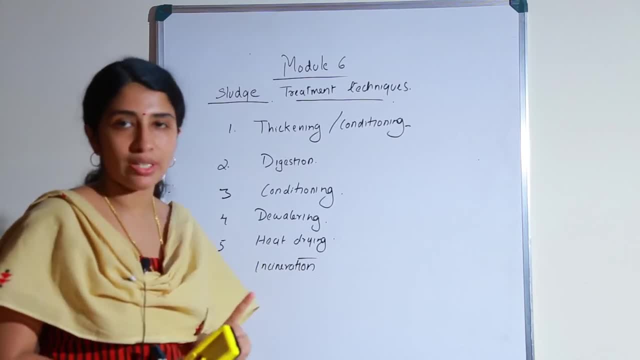 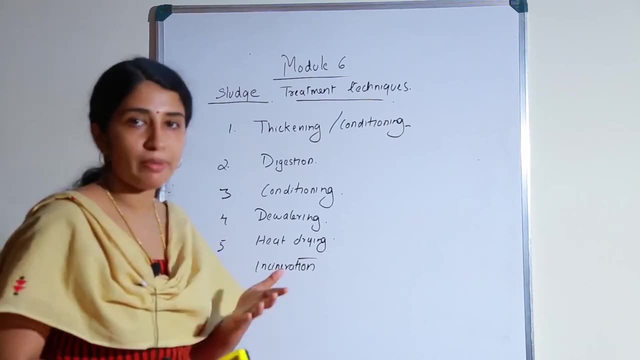 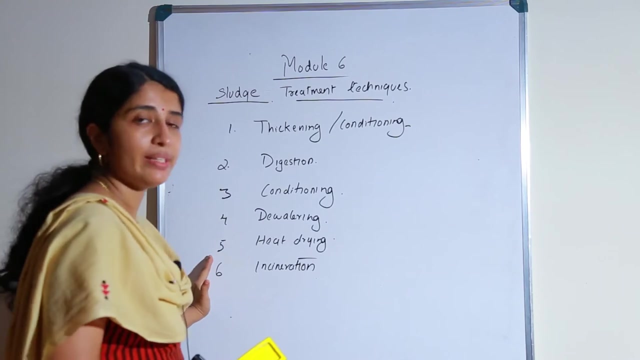 their aim, then they areIR important to see what they are giving. but those techniques are two. one is to reduce the moisture content, then to decompose the organic matter. these are the two aims or purposes of this different treatment techniques. so this is the order of treatment. 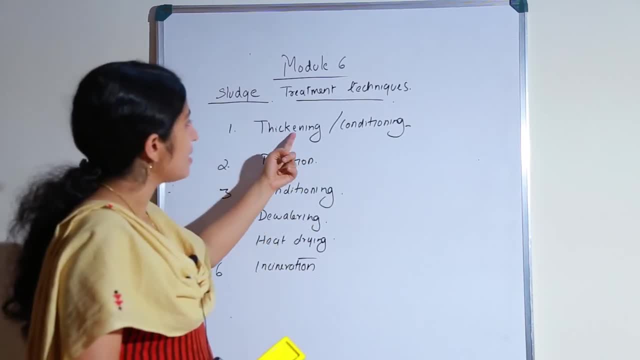 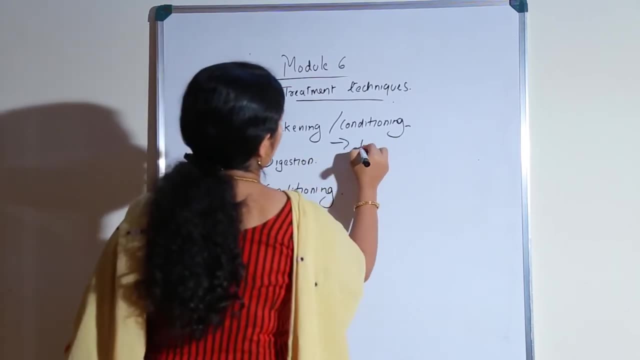 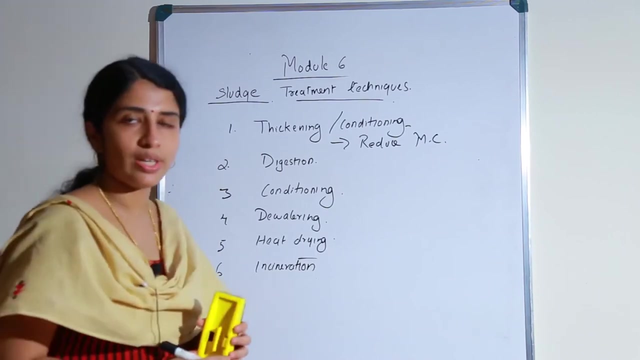 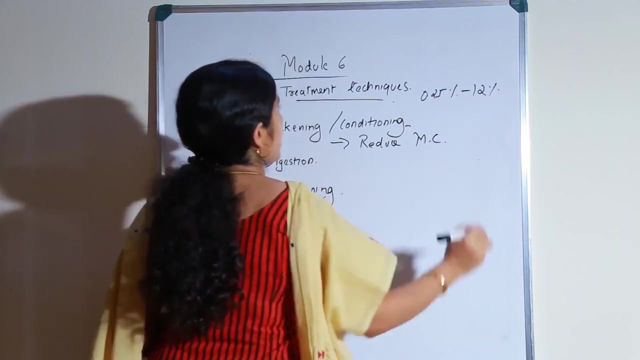 that we are giving for a sludge before the disposal. the first stage of treatment is sludge thickening or conditioning meant to reduce the moisture content of the sludge. as we are considering a sludge, it is containing only 0.25 percentage to 12 percentage of solids. the 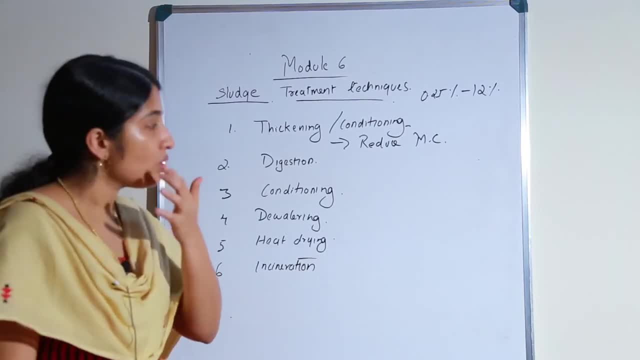 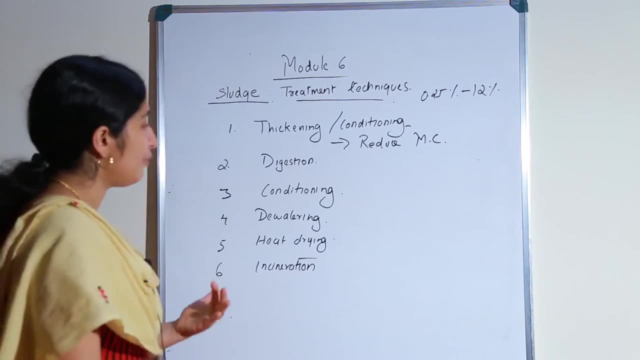 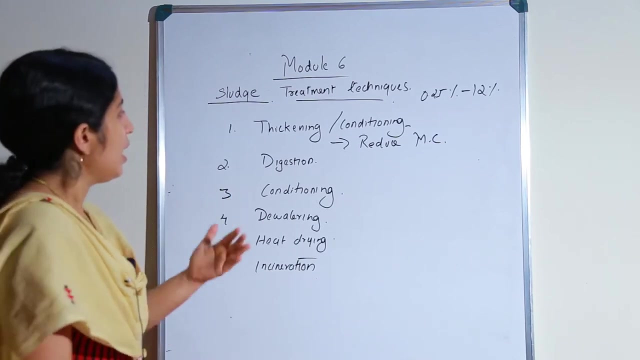 left percentage is for water. so this sludge is having a high amount of moisture content which needs to be reduced before the before we are disposing or treating the further process. at first we have to reduce the moisture content, which is really high for a sludge, so that 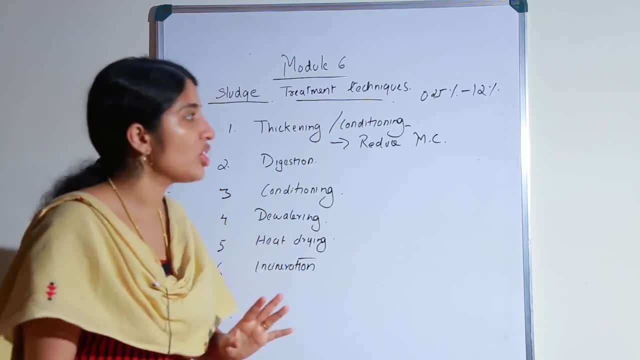 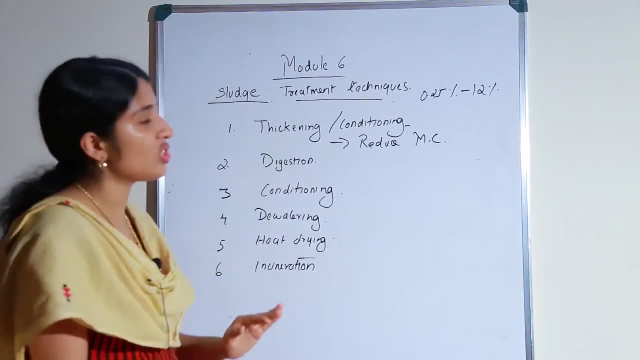 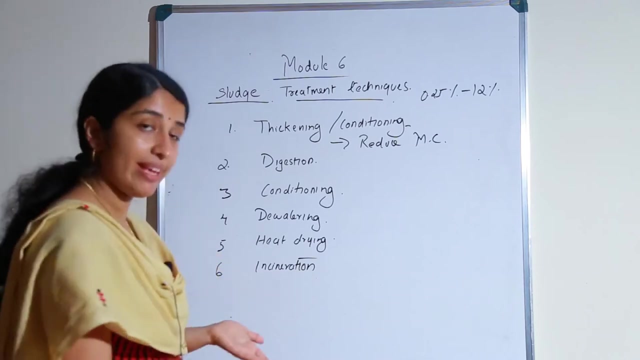 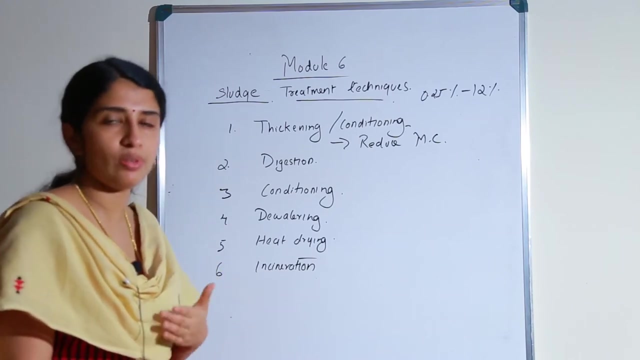 is called as thickening, sludge thickening or sludge conditioning. the next step is digestion- sludge digestion- sludge digestion means to decompose the organic matter present inside the sludge. it can be either aerobic process or through anaerobic process. the treatment system that we are used for digestion is called as sludge digestion. 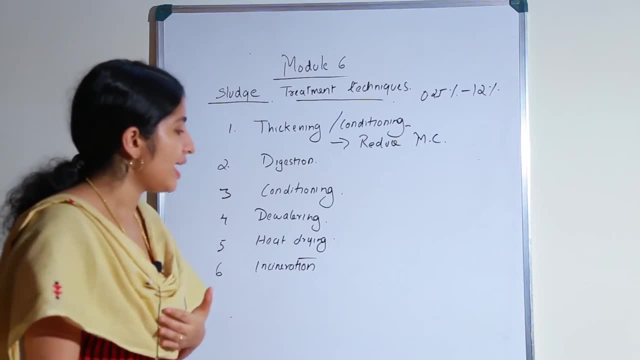 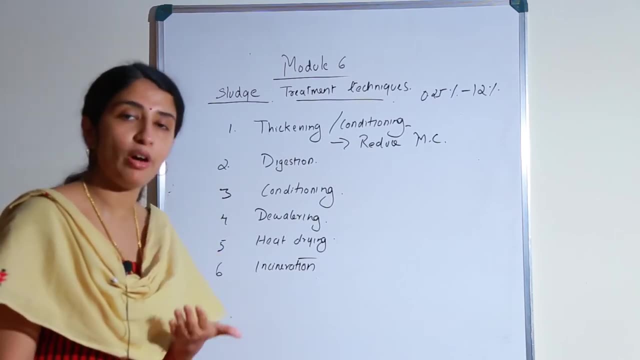 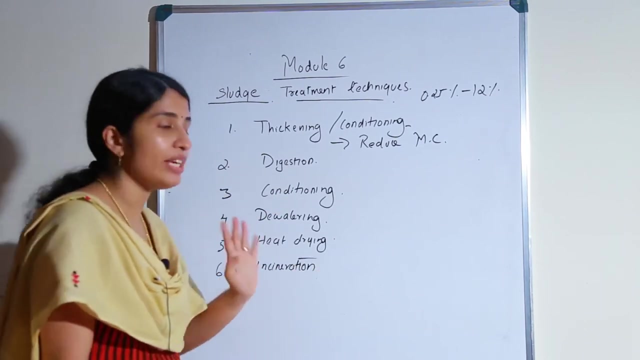 sludge digester. so through a sludge digester we can decompose the organic matter present inside the sludge. so that is the second step of treatment. then the third step is conditioning. conditioning means to prepare the sludge for the dewatering process, which is the next treatment step. 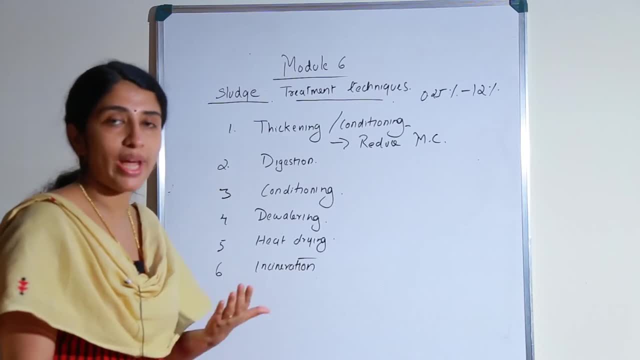 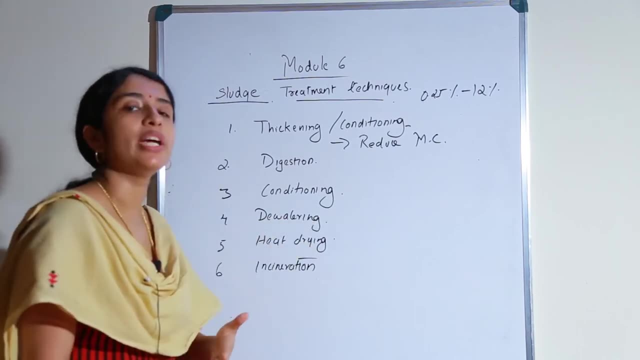 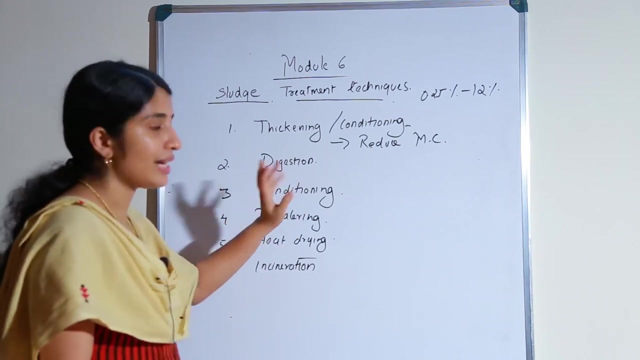 so conditioning means to enable or to enhance the drainability of sludge or to help the next process called dewatering, to make the sludge capable for dewatering process. so that is about conditioning. the conditioning is done with the use of different chemical conditioners. 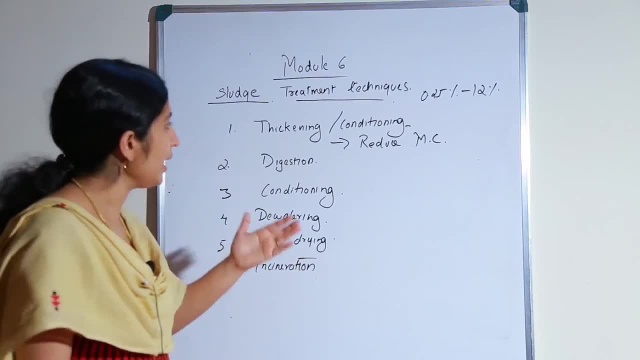 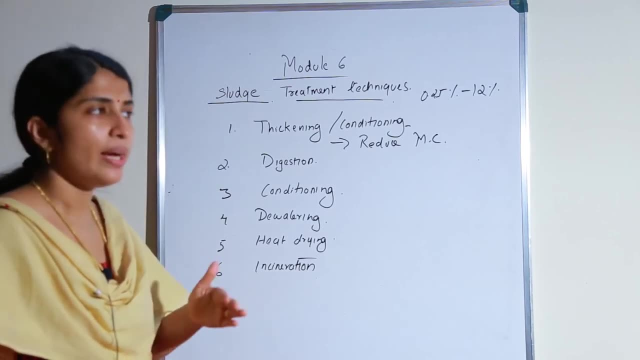 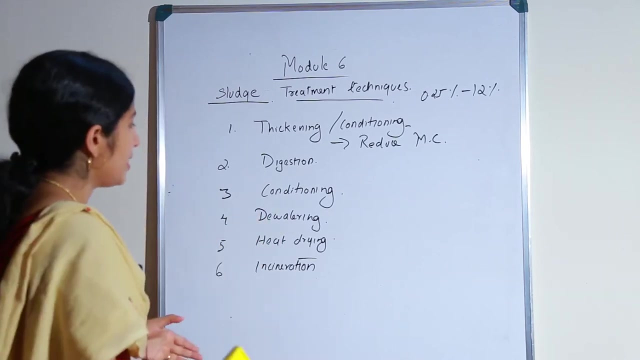 so that is about conditioning. next dewatering already in the thickening or conditioning stage itself, the moisture content will reduce up to 90 percent. still, there is moisture content which needs to be reduced. that is done using dewatering techniques, the dewatering system that we are used. 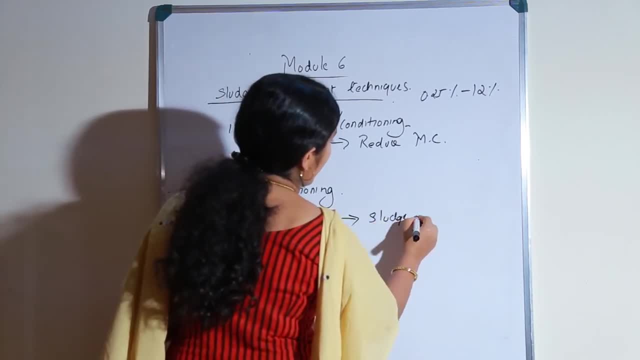 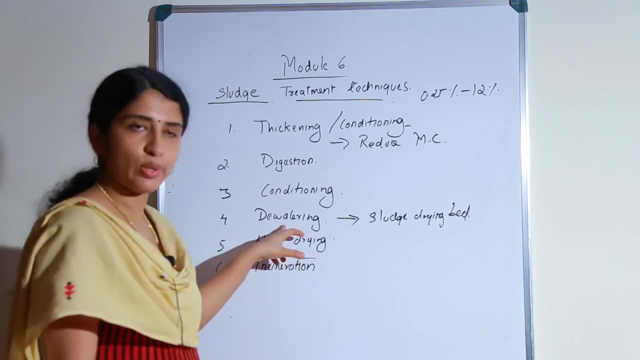 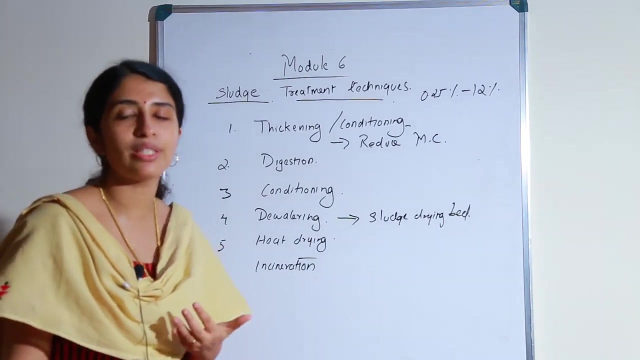 for a sludge is called as sludge drying bed. in a sludge drying bed we can dewater the sludge also in this process. in the dewatering process we can reduce the volume of the sludge and also to reduce the moisture content. along with the moisture content, the volume of sludge also get. 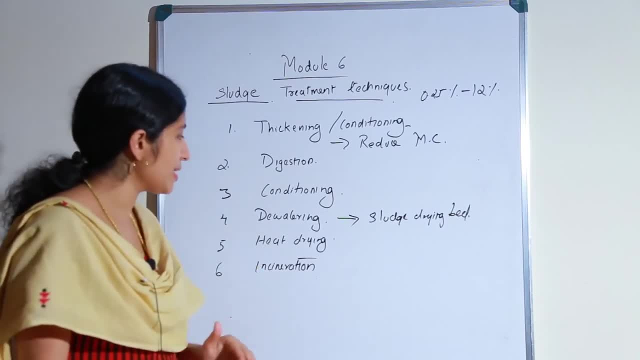 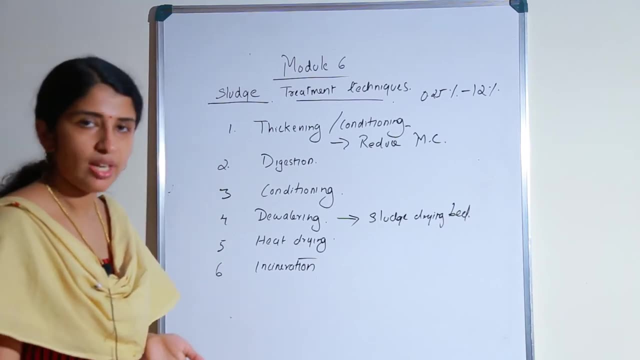 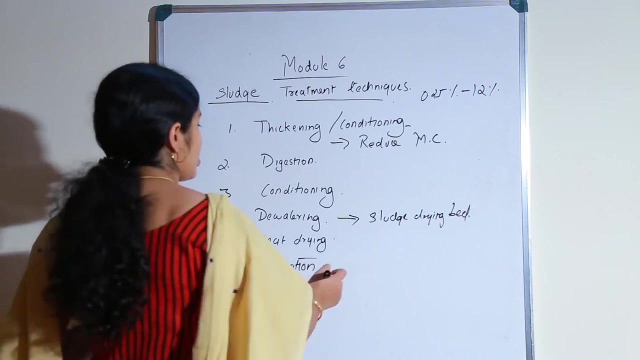 reduced in the dewatering stage. now the next step is heat drying in a rotary in or in a furnace. we will heat the sludge and the purpose of this is again to reduce the further moisture content still in the sludge, which is done in the safelyёт. this is a matter of heat drying and slicing. 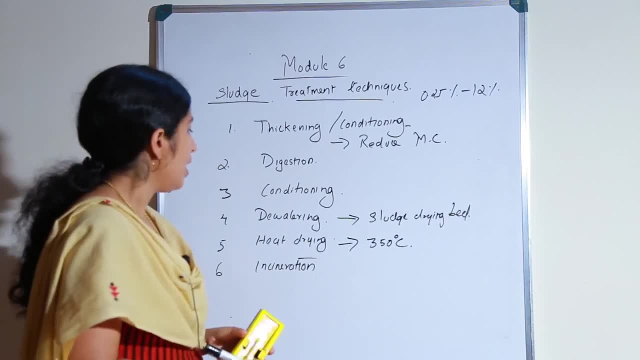 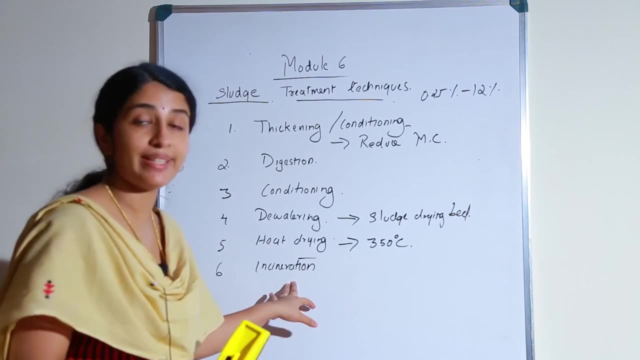 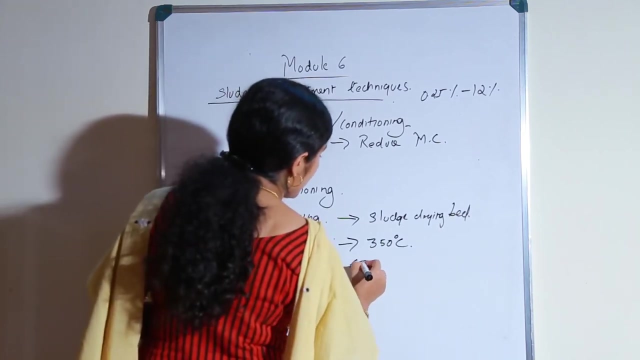 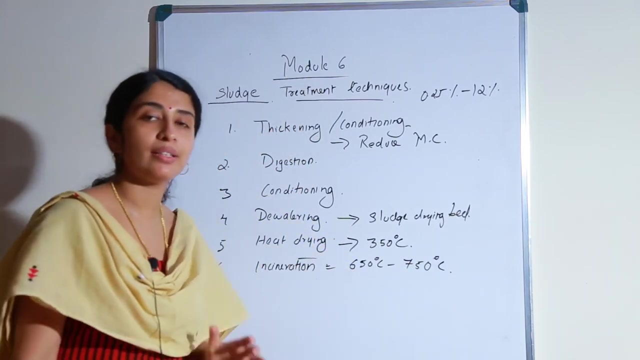 the sludge length at the temperature of moist on the edge of heat in the sludge. heat drying to the ability of vi teaspoon in the sludge hat is done at the temperature of three-fifty degree celieus. oozing in repairing are Celsius to 750 degree Celsius. at a really high temperature we will burn the. 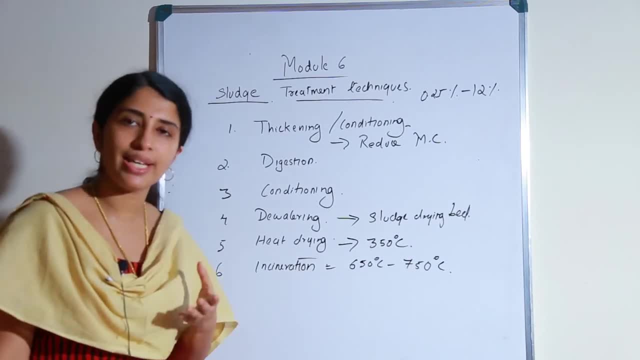 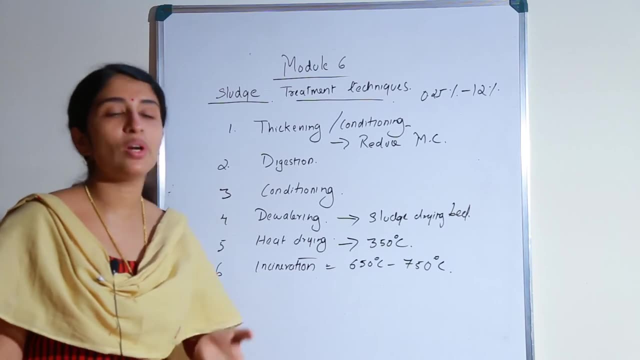 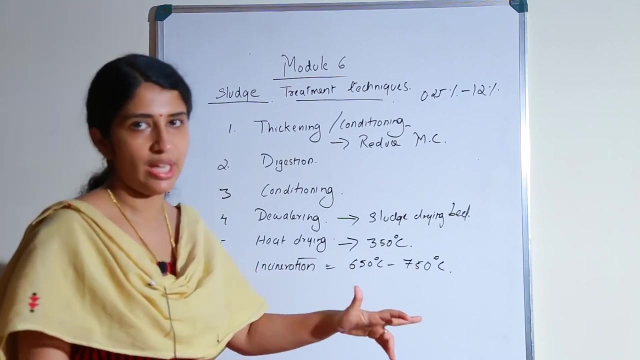 sludge. at this point of time the sludge is having very less amount of moisture content, which is removed through all this one to five steps, and also the volume. the total volume of sludge is very less. in that condition we can easily incinerate the sludge. if the sludge is having much higher amount of 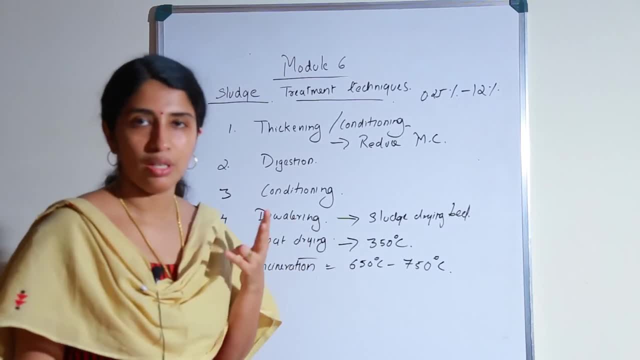 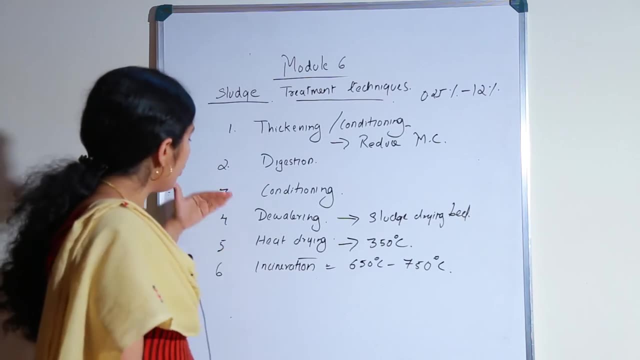 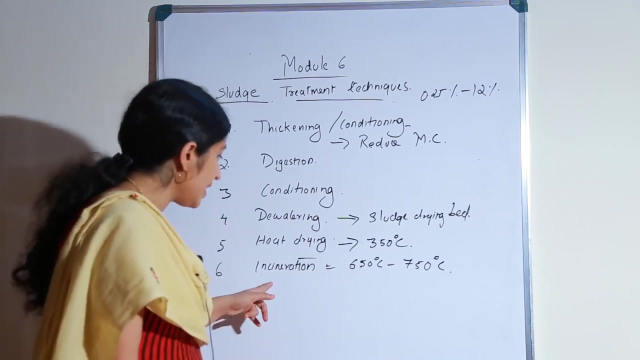 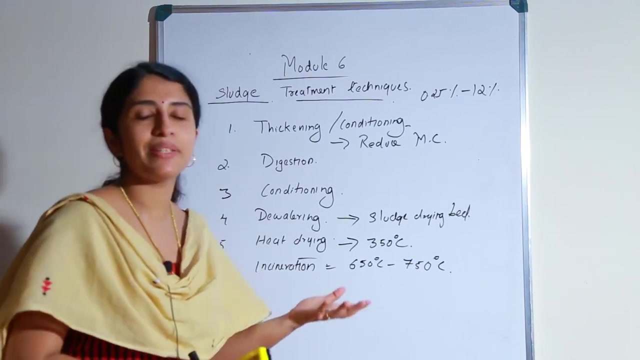 moisture content. incineration process is not. incineration process is difficult to carry out. so before that, through the one to five steps, we are removing the high moisture content of the sludge. so in incineration we will again remove or we will burn the organic matter or the microorganisms present inside the sludge. 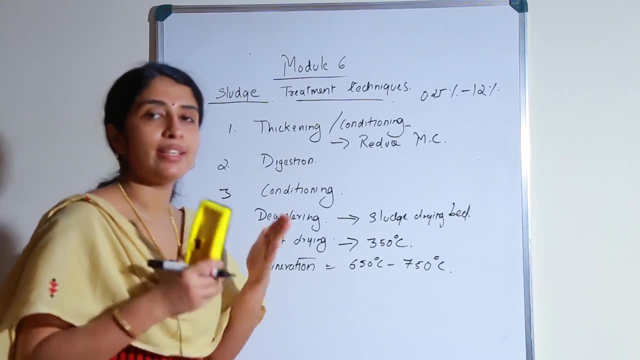 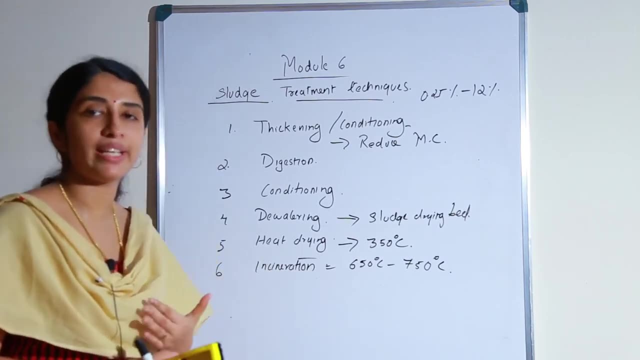 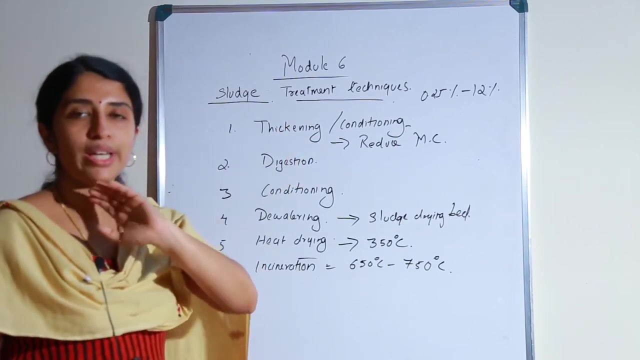 thereby make the sludge for a safe disposal. this is the final treatment technique. hope you understood different treatment techniques. once again, let's have a look. the first one is thickening or sludge conditioning, which means it is to reduce the moisture content of the sludge, and also one thing to remember is that there are several. 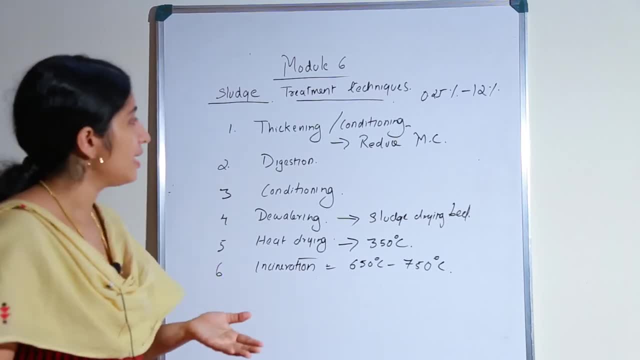 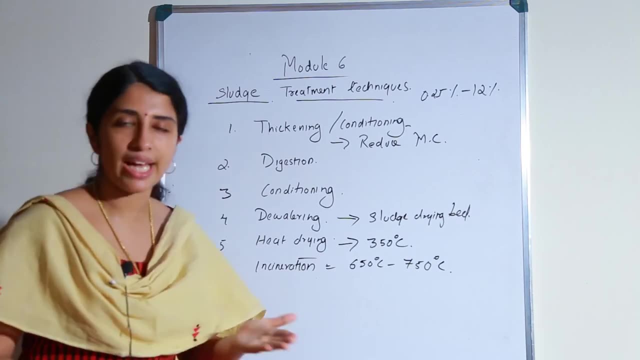 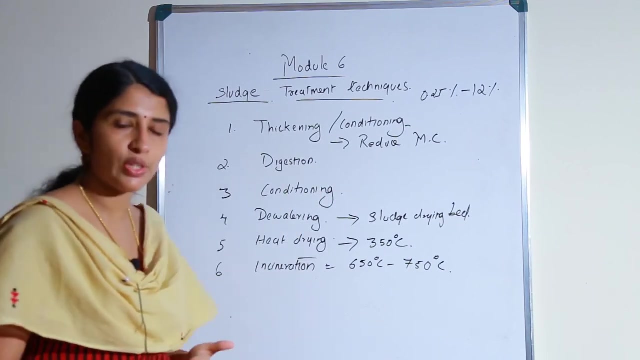 techniques or several methods of sludge conditioning or thickening. similarly, for each and every techniques, there are different types of techniques used. for example, in thickening we have gravity thickening, then flotation, centrifugation. these are all the thickening techniques that we are used, which we will see later. for 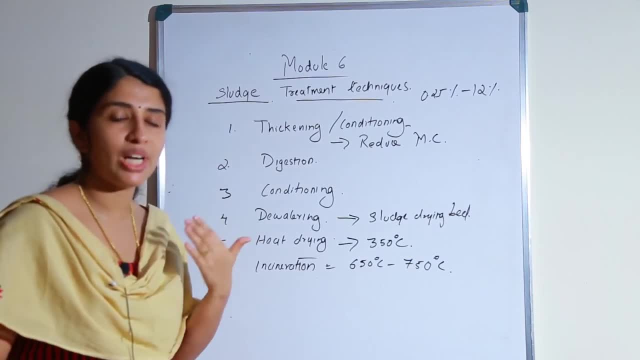 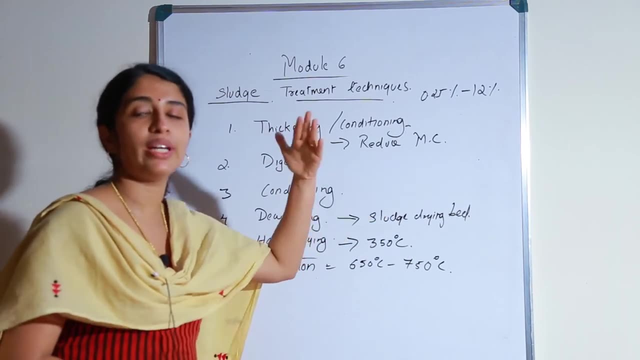 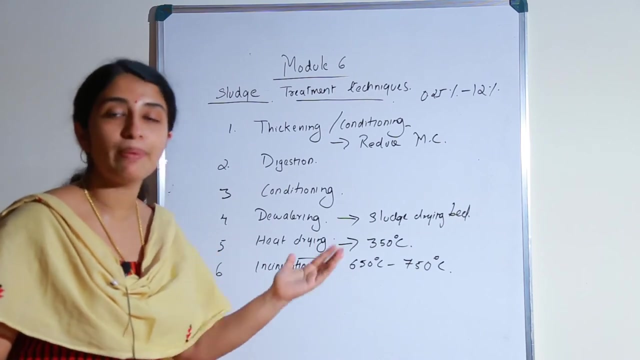 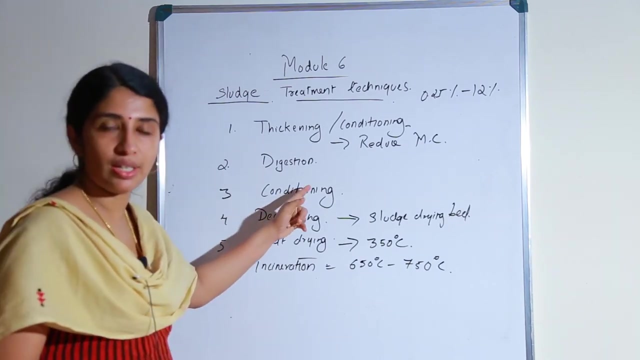 today we are dealing only with what are the various step, or what are the purpose of various step of treatment techniques. so thickening is for reducing the moisture content. second one is digestion. digestion means to remove the or to decompose the organic matter present in the sludge, either aerobically or anaerobically, then conditioning, which this step will enhance. 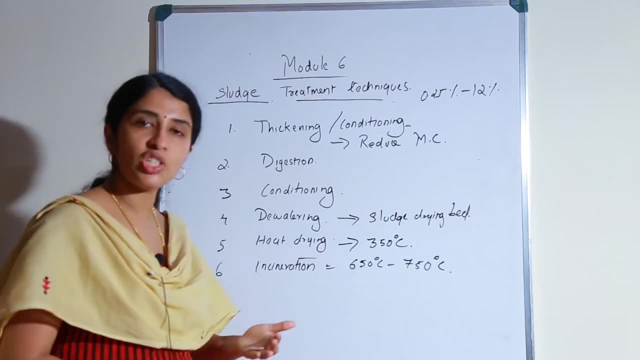 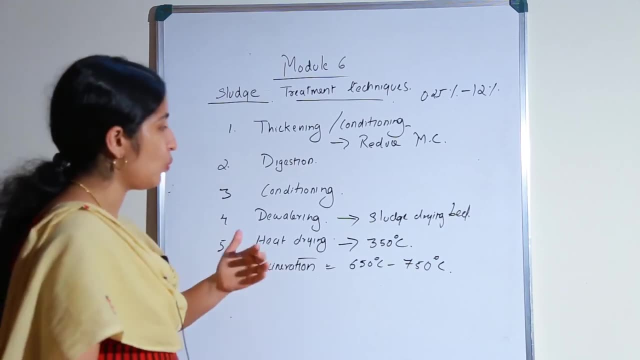